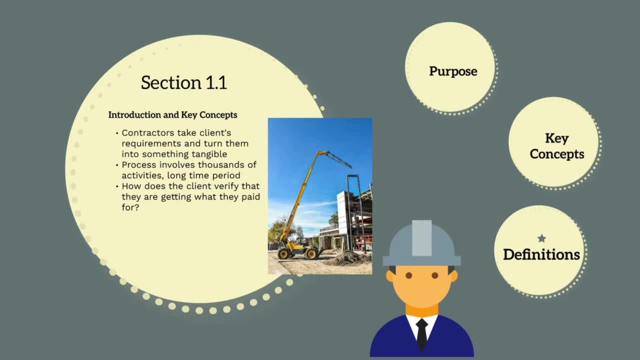 quality management. We'll talk about its purpose, the key concepts to understand and some definitions. When we think about what a construction project actually is, it consists of a client defining what they want and engaging and paying a contractor to turn it into a reality. 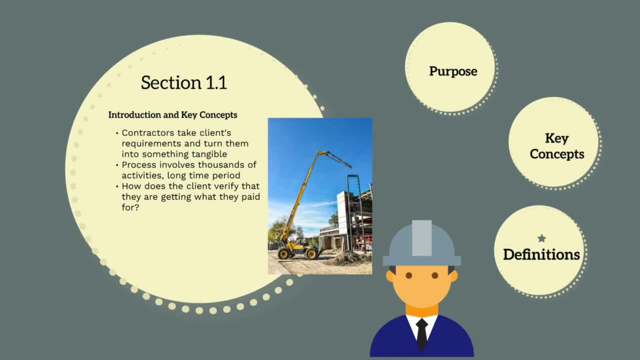 This process can take years, involving thousands of activities and steps, and an important question to ask is: how does the client actually verify that they are getting what they paid for? Well, I'm glad you asked. That's where construction quality and completions management comes in. 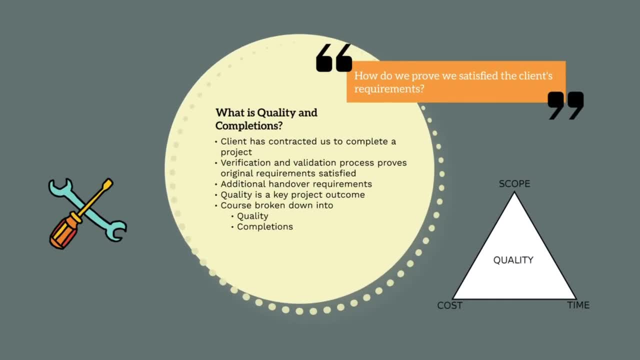 The easiest way to think about this topic is about providing, is about proving that we have satisfied the client's requirements. Working for a contractor, a client is paying us to deliver a project for them, Be that a new bridge, water treatment plant or hospital, Depending on the specific contract. 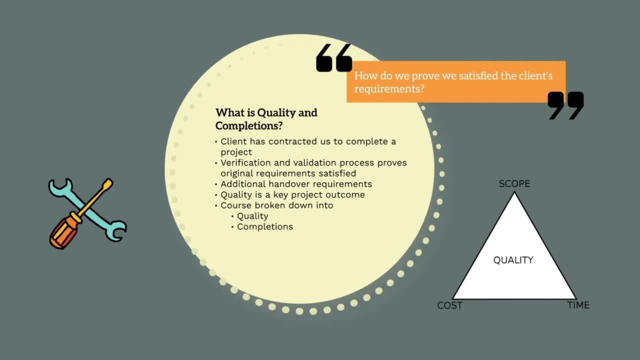 model chosen. a client will have defined their requirements and it is our responsibility to deliver it for them. But how can they be sure they're getting what they paid for? Well, that's the purpose of quality. Quality is the verification and validation process. we 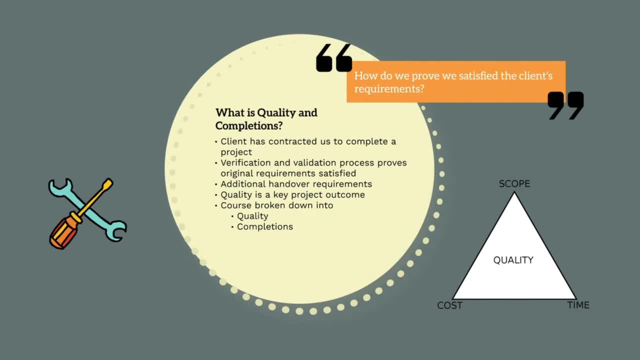 go through to prove these original requirements have been satisfied. A really easy example to reinforce this is: imagine we're contracted to build a hospital. As part of the project requirements, we have to provide adequate lighting in each room to a level of 80 lux. 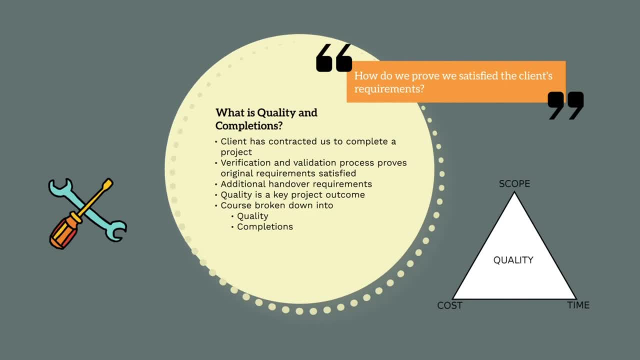 a measure of lighting levels. Therefore, as part of our quality control process after the lighting is installed, we'd go through with a lux meter, a tool that measures light and prove each room achieves the requirement of 80 lux. if we go back to project management basics, 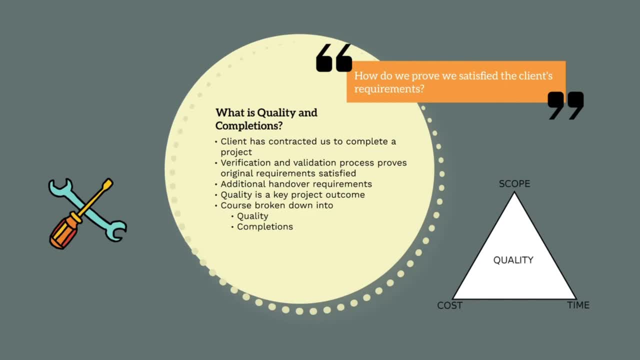 quality actually forms part of the fundamental project management pyramid. to the right hand side, you can see that the project management pyramid showing us the fundamental project outcomes: scope, which represents what, what we actually deliver. time, which represents the overall project duration. and cost, which represents the overall project budget. 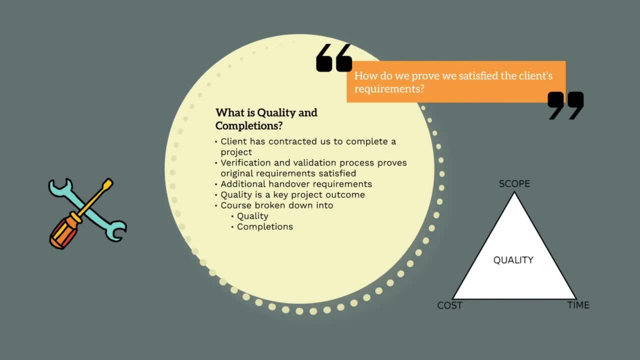 quality is shown in the area between them all. basically, what it means is that we cannot adjust scope, cost and time without affecting quality. if we try to do more scope with the same budget and time frame, we'll reduce the quality standards. if we try to deliver the same scope faster and cheaper, 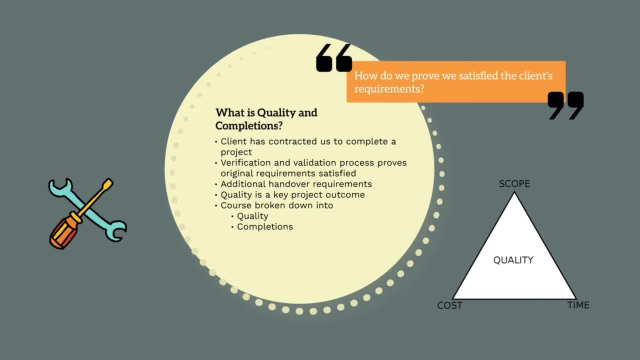 it will again lower the quality of the works. quality is a really fundamental concept to understand on your engineering journey. on top of simply proving what we've delivered matches the original project requirements, the client will have additional requirements around finishing and handing over the project. the management of these components is referred to as completions management. 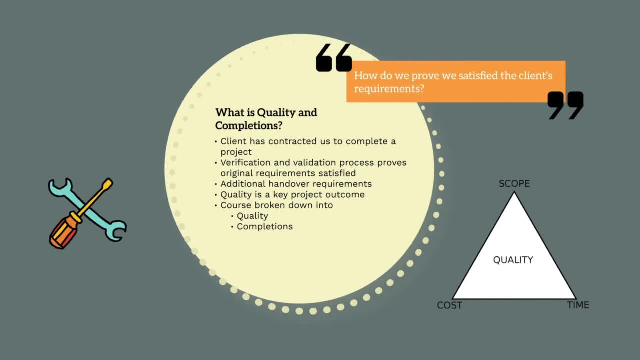 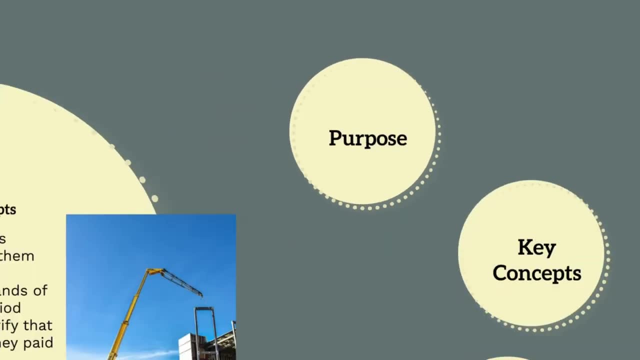 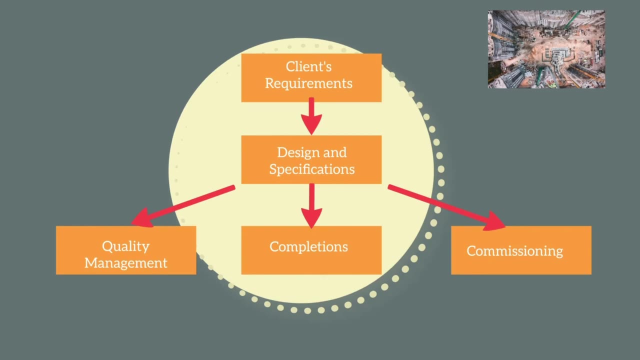 while they are slightly different, they are tightly, tightly related, and that's why they're going to be covered under this same course. let's now look at these key concepts as in a diagrammatic form, so we can really understand their relationship, starting at the top, as we discussed a 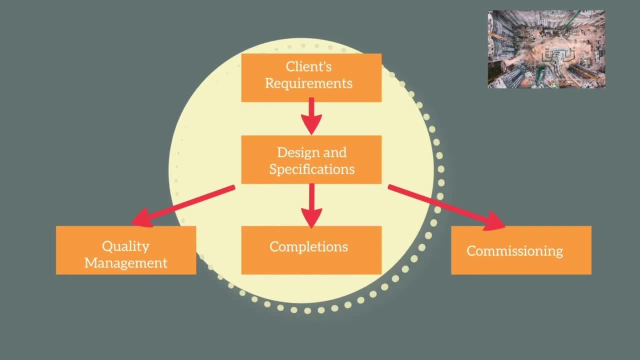 construction project exists in the first place to satisfy some need or objective of the client. these are the client's requirements. so a client may want a new water treatment plant built. they may require it to process a certain amount of water, operate with a certain reliability, fit on a block of a certain size land, and these requirements are typically captured in a project. 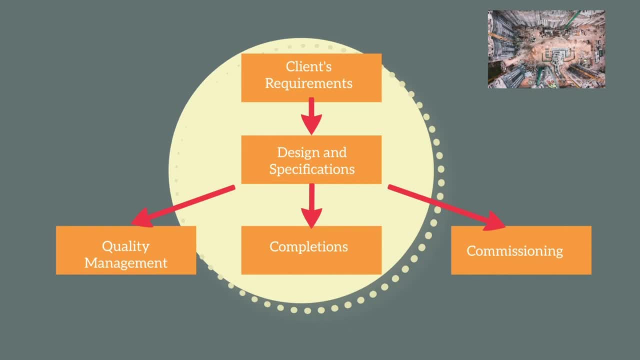 requirements document, such as a specification, standard or concept design. a design consultant will take these requirements and develop the project design. the design consists of the drawings and specifications that describe in detail what is to be constructed. so, while the original project requirements may detail the need for a water treatment plant that can process a certain amount of water, the design tells the 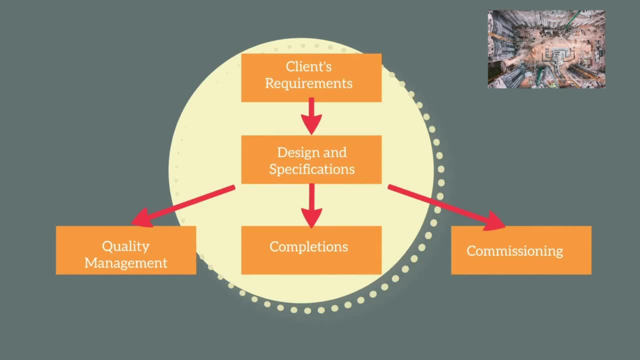 contractor exactly what requirement they need: need to order where the equipment is to be installed, the walls and the roofing details the equipment will sit in, and so on their need. there needs to be sufficient detail in the design so somebody can actually go out and construct it critically. 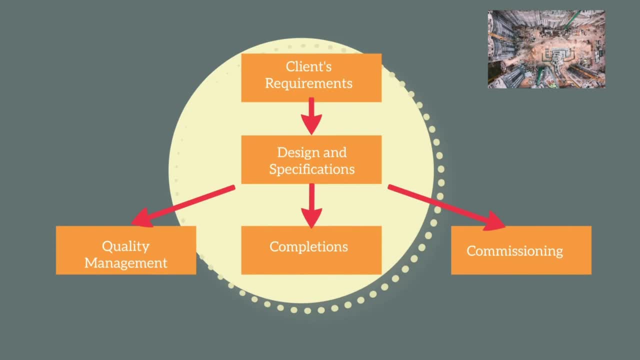 important to understand, though, is that what the design is telling the contractor to build needs to capture all of the client's requirements. this is super important to understand and reinforce. during the design process, the client will review and sign off the design, and there will be checks in place to ensure all of the project requirements are captured in the design. 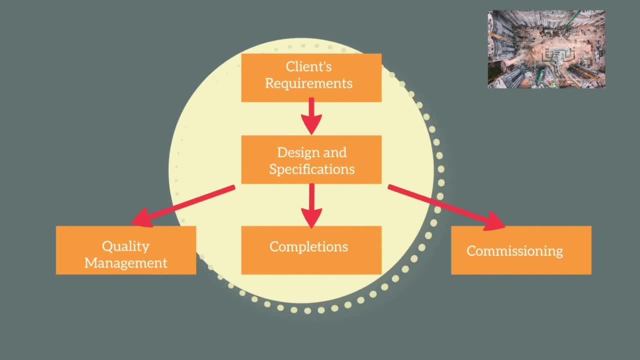 depending on the contract model used the client would. depending on the contract model the client uses to engage the contractor, will depend on whose responsibility it is to produce the design. so under design and construction contract, the contractor will engage a consultant to deliver the design, while under a construct only. 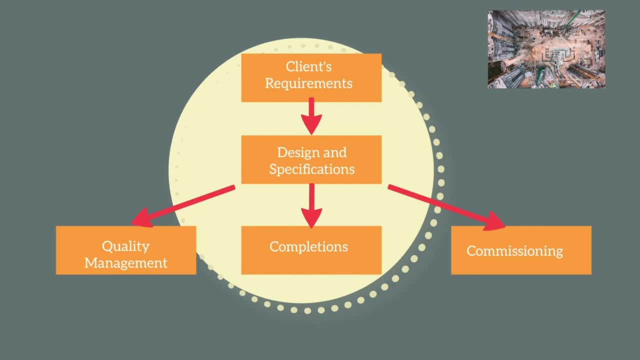 contract, the client will develop the design themselves. therefore, quality on construction projects is focused on. it is focused on proving that what has been built matches what was detailed in the design. where possible, the quality process will attempt to evidence that the original client's requirements have been met, but usually this is more difficult in practice. the focus is on proving what has 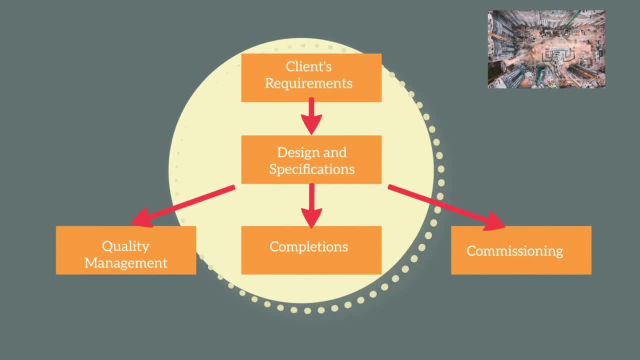 been constructed matches the design. it's important to note that proving that the design matches the original client's requirements is not part of the scope of this course. as this course focuses on construction quality management, That falls under the topic of design management and will be covered. 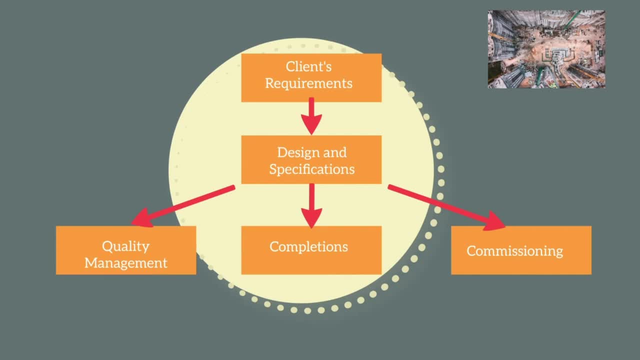 in a separate Engeloan design management course. Completions management focuses on the handover of the finished product back to the client. The client will have specific requirements relating to the handover of the project. For example, the contractor may be required to. 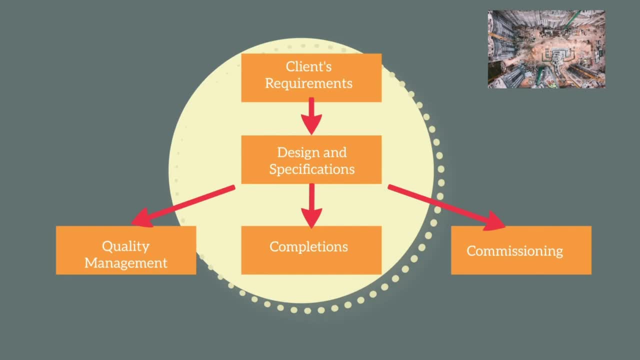 provide spare parts, warranties, training and so on, depending on the project particulars. The understanding, management and delivery of these requirements is completions management. Finally, commissioning is a testing process largely applicable to mechanical, electrical fire and other process systems where the delivered product is function tested against. 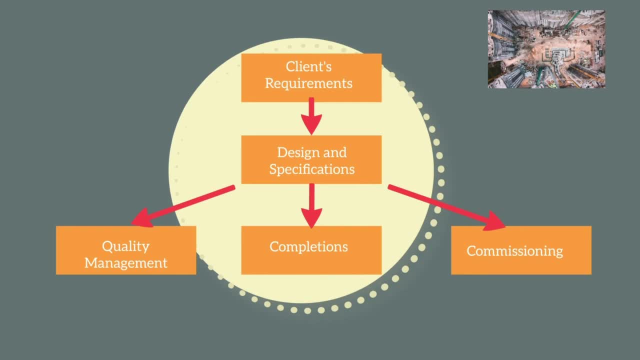 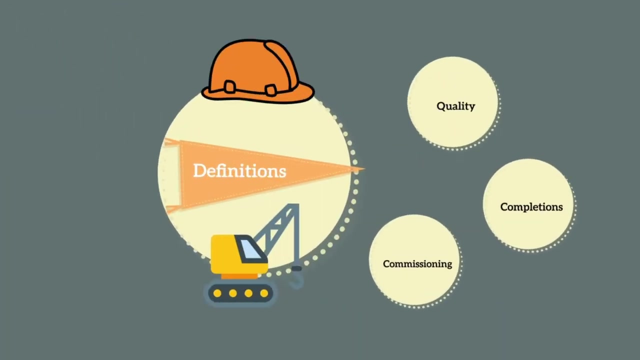 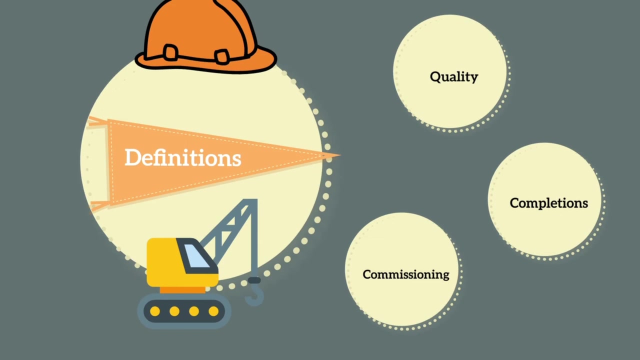 the original requirements. I've included commissioning under quality and compliance in the video description. Now we've introduced the concepts, Let's now try and lock in some definitions for these terms. We'll look at how some of the terms are defined in other resources as well. 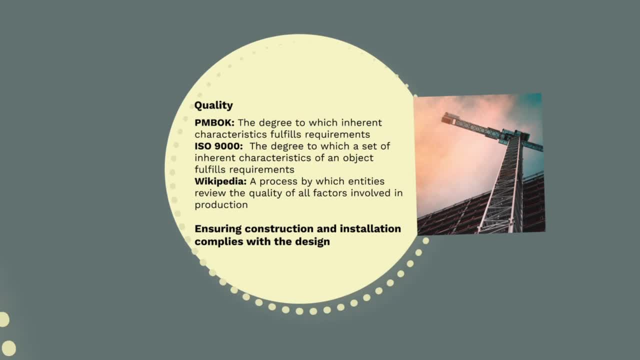 Starting with quality. the project management body of knowledge defines quality as the degree to which inherent characteristics fulfil requirements. The PMBOK is an awesome tool for understanding project management at a fundamental level, and I would strongly recommend completing a PMBOK course. PMBOK focuses on all facets of project management, not just construction management, so it's 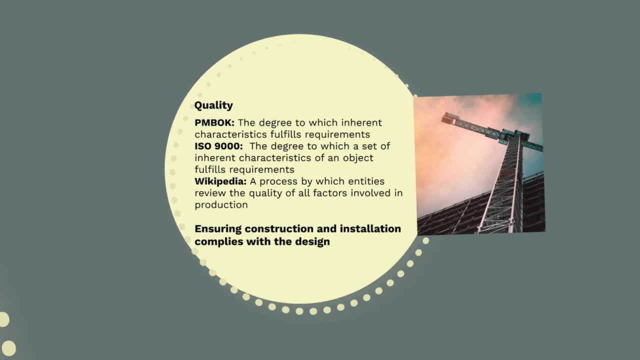 not super specific. ISO 9000 is the widely accepted source of truth on quality management. It's used by all sorts of industries, including maintenance, construction, product development and IT. They define quality as the degree to which a set of inherent characteristics of an object fulfils requirements. 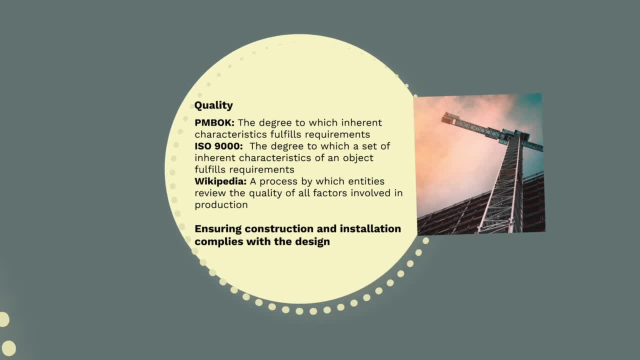 And finally, we have Wikipedia. They define quality as a process by which entities the quality of all factors involved in production. In short, all these definitions are correct and useful. I just want to highlight that the unique thing with construction quality is that the focus is on proving that the installation 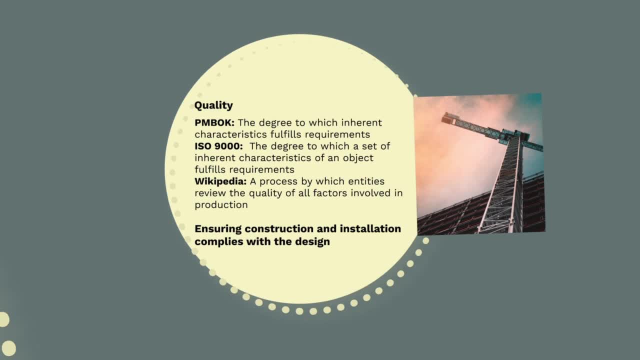 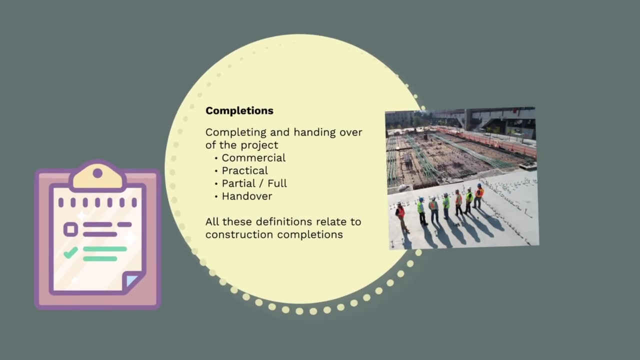 complies with the original design. The design is meant to encapsulate the original requirements. In summary, the most useful and functional definition of quality that I can come up with is ensuring construction and installation complies with the design. Completions management covers the final project handover to the client. This means once construction. 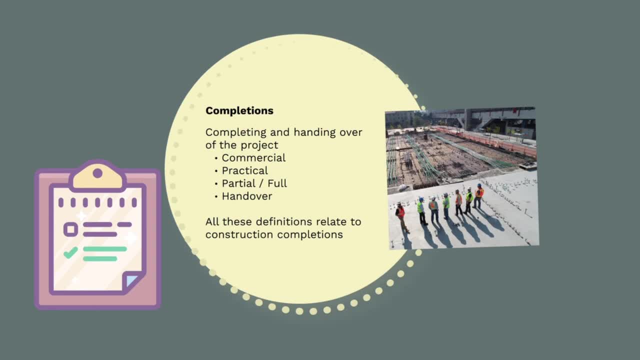 is complete, we take our padlocks off the gate, pack up and give the keys to the client. The process and management of the specific project is the most important part of the project. The process and management of the specific project is the most important part.